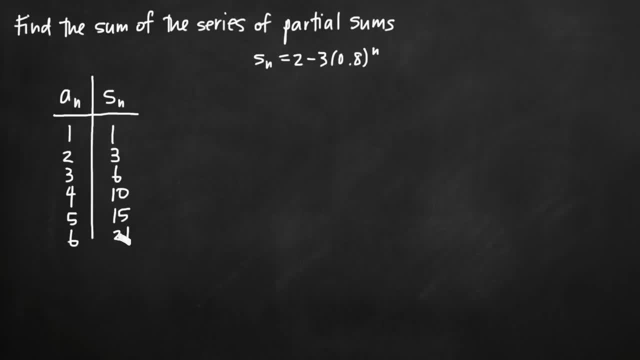 would be denoted s sub n as one, three, six, ten, fifteen, twenty-one. So that's the difference. And in this particular case, obviously, we're going to have a series of partial sums of the series, a sub n. 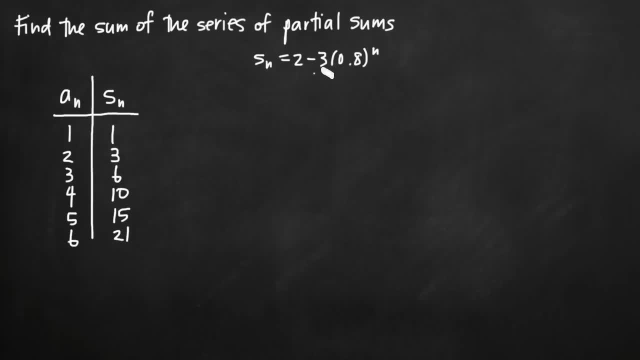 Obviously, we have the series of partial sums s sub n in this equation here. Now, how do we find the sum of the series of partial sums? Well, what we need to know is that what we're really talking about here is the infinite sum of the series, a sub n, right? 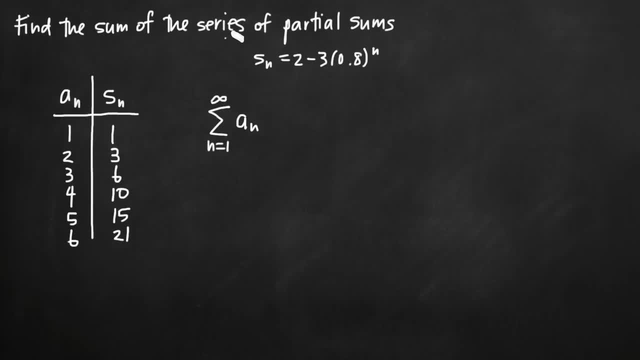 from n equals one to infinity. That's the sum of the series, But we're dealing here with partial sums. Well, it turns out that the sum of the series as we take n out to infinity is just equal to the least sum of the series. 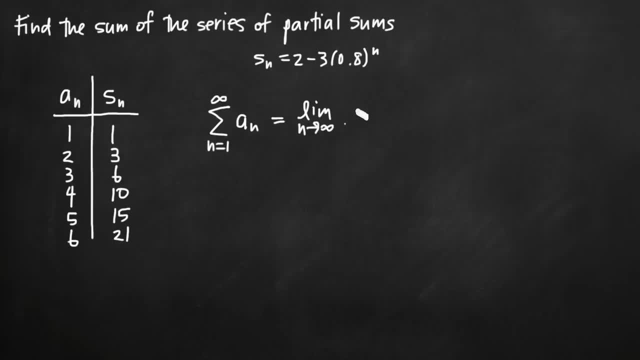 So what we're going to do is take the limit, as n goes to infinity, of s sub n, the series of partial sums. So this is a convenient tool for us. This is a convenient equation for us to use often, because if we have the series of partial sums here s sub n, we can just 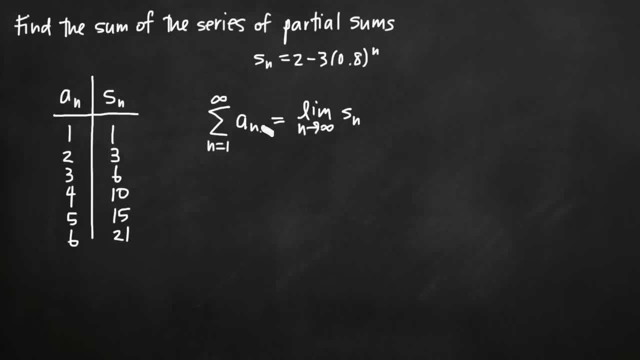 take the limit, as that series goes to infinity, and it gives us the sum of our original series. So what we're going to be evaluating here is the limit, as n goes to infinity, of s sub n. Now, to do that, in place of s sub n, we can just plug in our equation here, So we'll get. 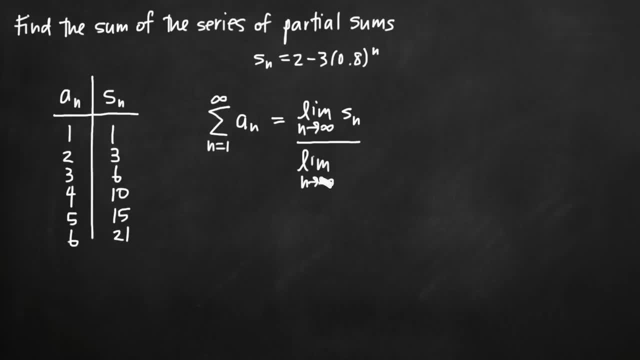 the limit, as n goes to infinity, of our equation: 2 minus 3 times 0.8 raised to the n power. Now, if we essentially plug in an infinite value here for n, if we plug in an extremely large value for n, what we find is that this quantity here, 0.8, raised to the n power, 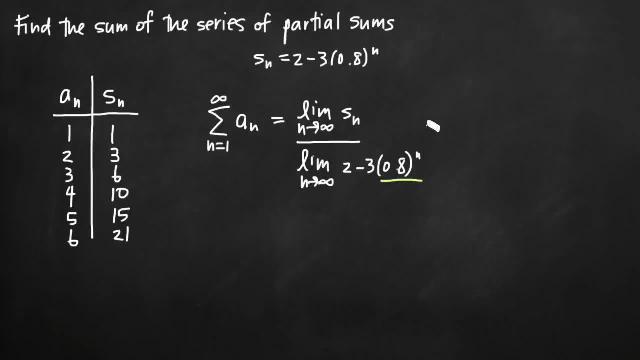 continues to get smaller and smaller and smaller and smaller, Because if you take 0.8 and you multiply it by itself, what you get of course is 0.64, which is a smaller value than 0.8.. If you multiply it again by 0.8,, 0.64 by 0.8, or in other words, 0.8 cubed, 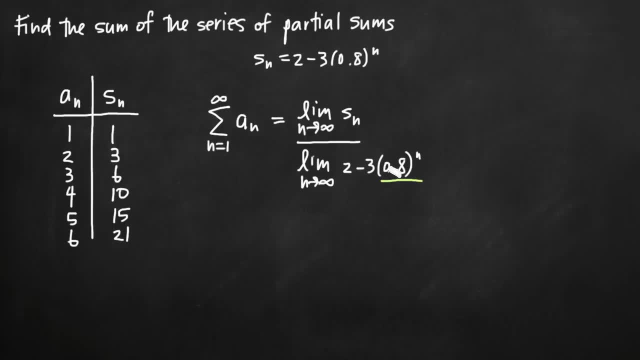 you get 0.512.. The value continues to decrease and get less and less and less and less. So what we can say is that, as n goes to infinity, of s sub n, we get 0.8 raised to the n power. So what we're going to do here is take the limit, as n goes to infinity, of s sub n and we're going to multiply it by 0.8.. If we take 0.8 and multiply it by 0.8, 0.8 to the.